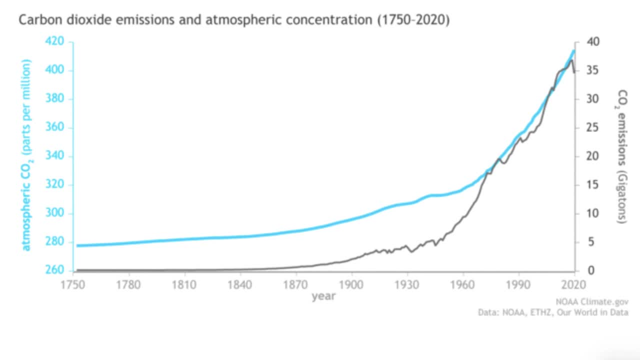 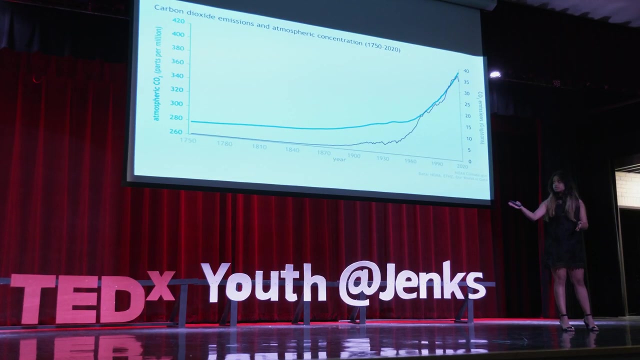 dioxide emissions. This graph, made from the NOAA, which is an organization comprised of climate scientists and academic institutes from around the world, made a graph that represents 1750 to 2020 atmospheric carbon dioxide emissions. As you can see, the blue line atmospheric 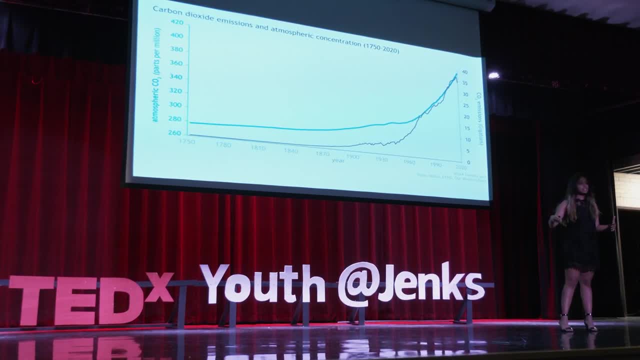 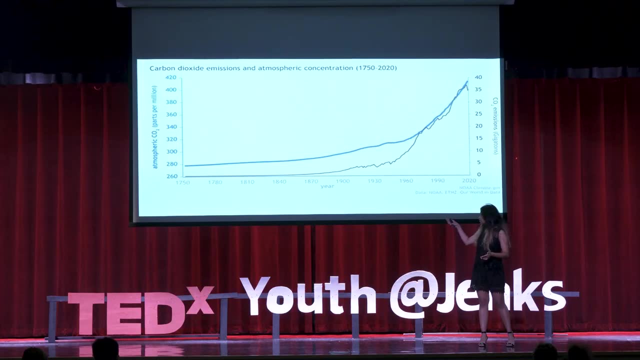 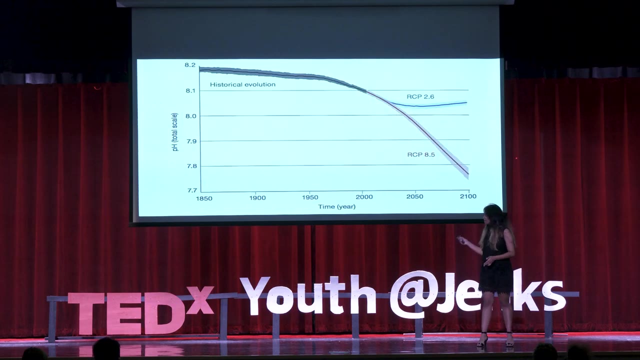 carbon dioxide and gray line, which is the carbon dioxide emitted from the ocean is emitted from us, rises simultaneously And in between 1840 and 1870, you can see there is a change in. there's a rise in carbon dioxide emissions And along with that pH of the 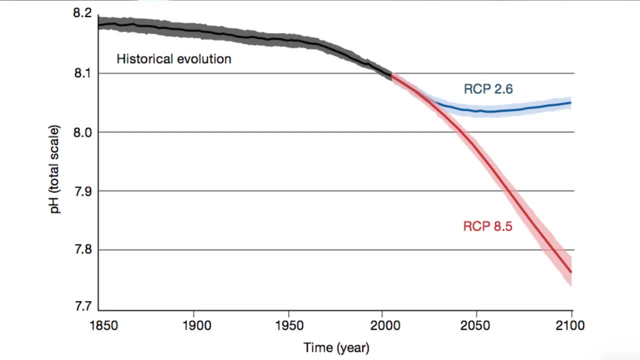 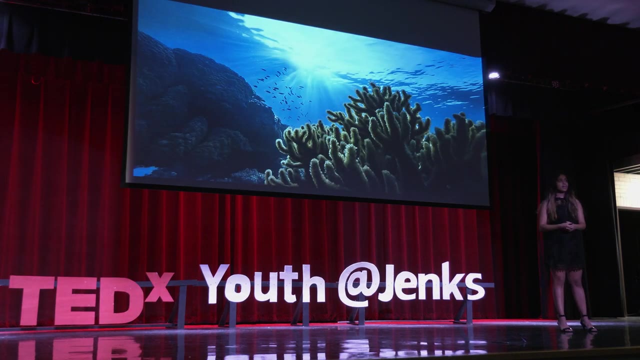 ocean has reduced. This graph shows past, present and future predictions of ocean chemistry. And as carbon dioxide rises around 1850, you can see pH of the ocean has reduced. And as carbon dioxide rises along 1850, the pH of the ocean reduces, So you can see pH of the 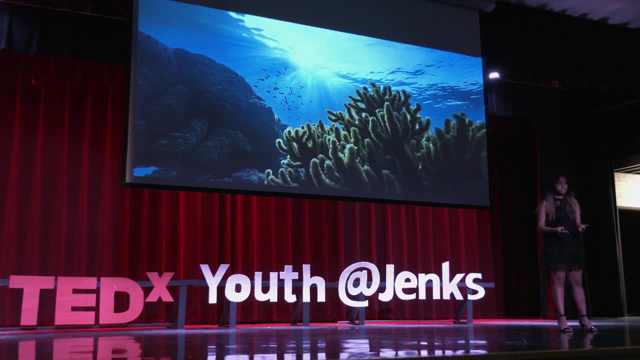 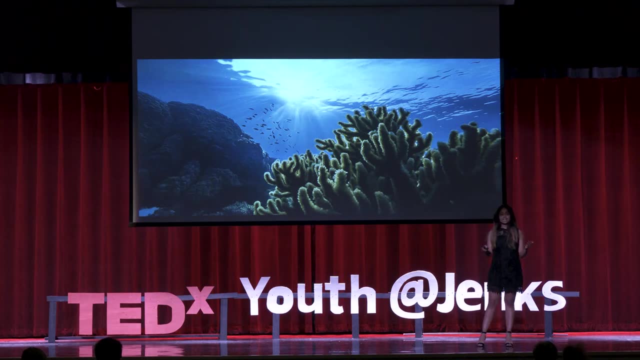 ocean is higher Now. this is ultimately because of how carbon dioxide dissolves into our oceans due to photosynthesis, And it was deemed that this phenomenon would be a natural solution to global warming, as this natural store would reduce the carbon dioxide in our atmosphere and would reduce 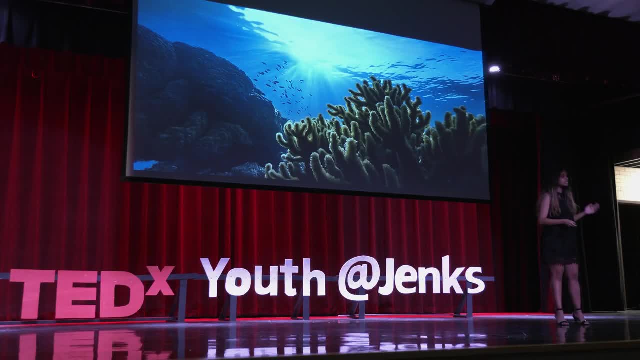 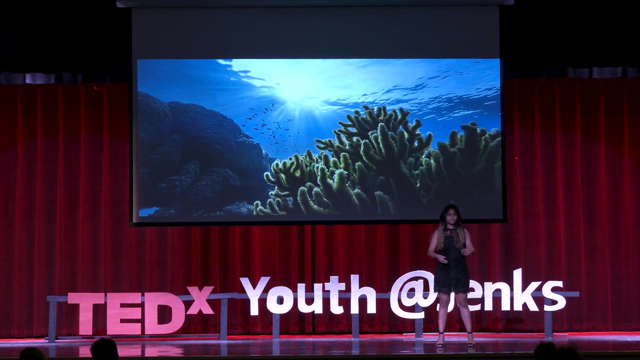 climate temperatures from rising, But when seawater combines with carbon dioxide, a chemical reaction occurs that ultimately reduces the ocean pH. As high schoolers, you probably think that this phenomenon has no effect on us, since we don't live by a beach, but ultimately, ocean acidification affects calcium organisms and carbon. 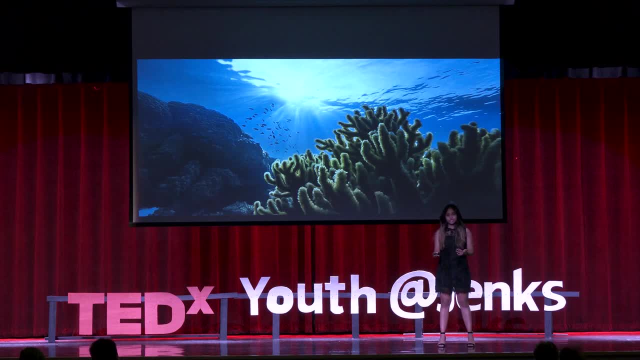 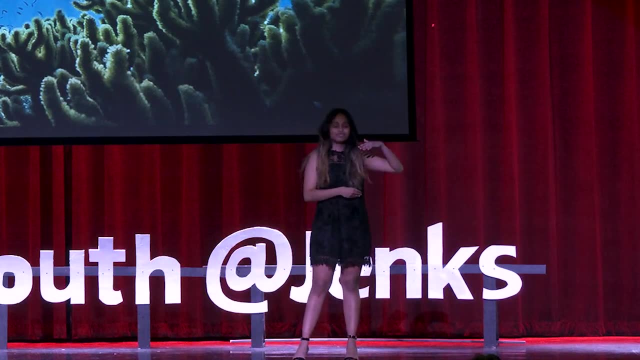 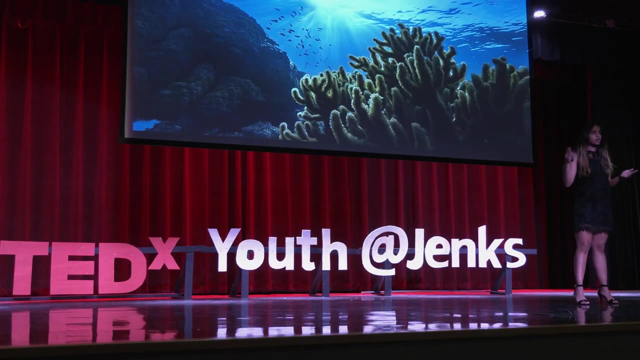 based shells, such as oysters and sea urchins- basically any organisms with shells- and slows their growth and dissolves their structures. This affects organisms higher up in the food chain that feed on these organisms. It can affect the commercial fish stock and eventually lead to job loss. Now the main. 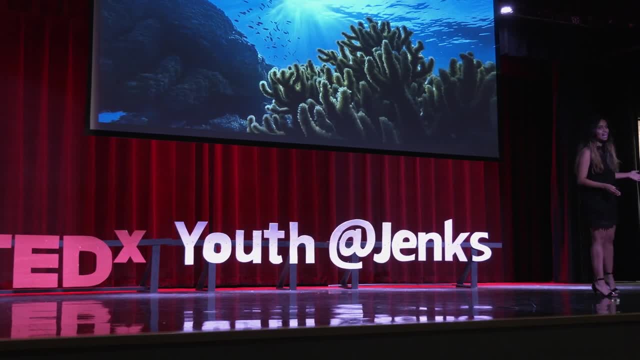 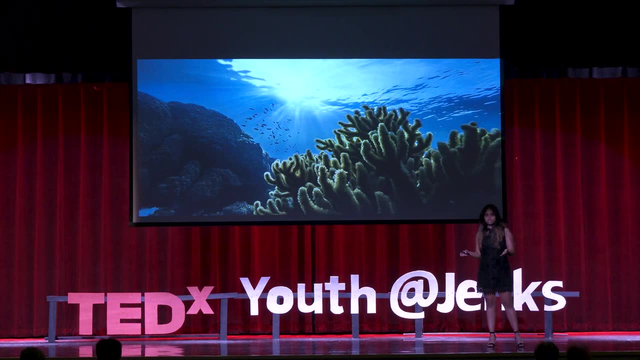 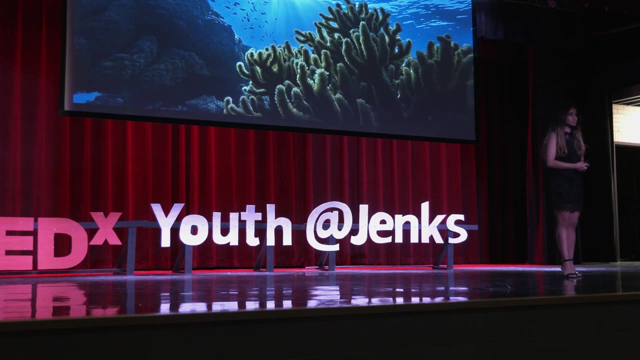 goal in tackling ocean acidification ultimately comes down to reducing our carbon dioxide emissions. By holding manufacturers and producers accountable to carbon dioxide emissions, we could limit the harm in marine life. And I know, like I said, we're all high schoolers and we don't have time. 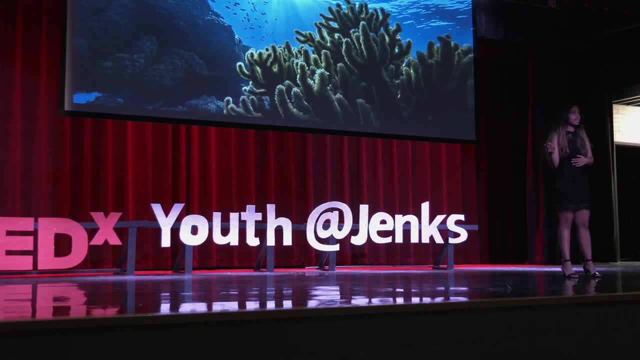 or we don't have the resources to do that, but we do have the resources to do that And I know, like I said, we're all high schoolers and we don't have time or we don't have the opportunity to go to court and protest and protest that these 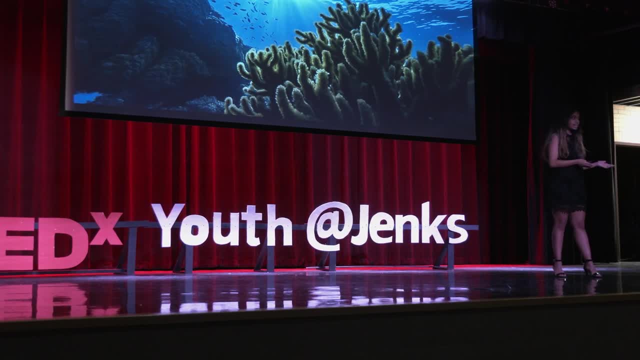 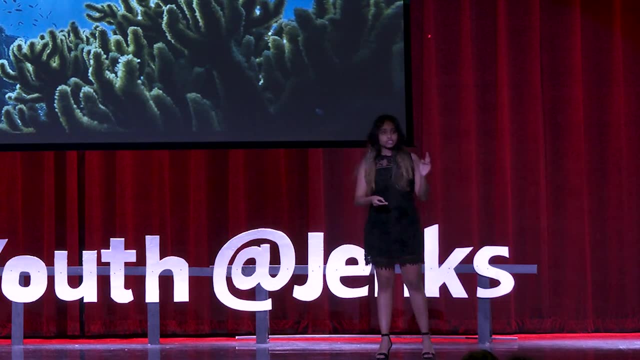 manufacturers are emitting these carbon dioxide, but it's not only them that emit CO2.. Every day in our lives we emit carbon dioxide into the air. A two-mile car trip produces two pounds of carbon dioxide into the air. Ultimately, we could ride our bikes instead or walk to the park instead of. 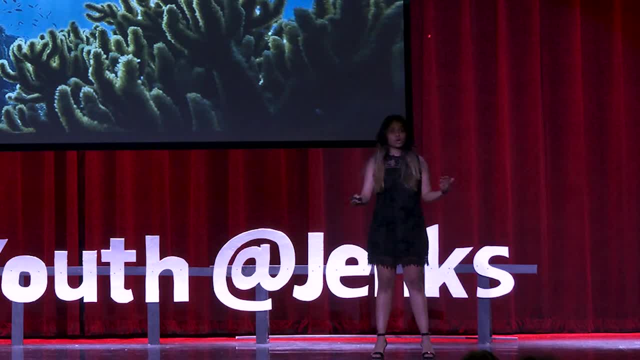 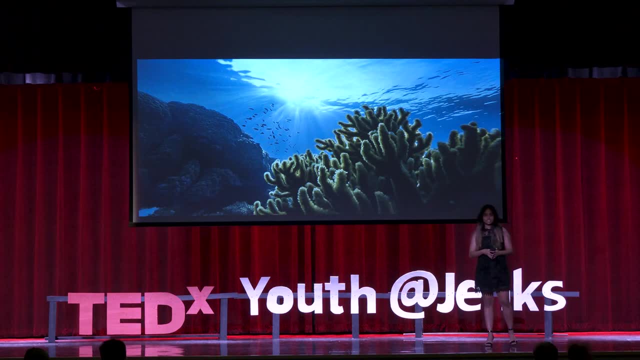 taking our cars, or even carpool, to places where we wanted to go- to the beach. We wanted to go with friends for a long road trip. Now, ocean acidification is usually hidden by the impacts of carbon, carbon dioxide, usually referred to as the doppelganger of global warming. because of how both processes are, 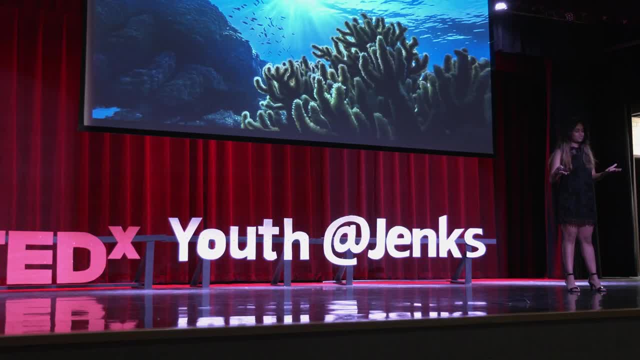 contributed to global carbon dioxide emissions. But since, even if awarenesses of this phenomenon is reduced low, the scientific evidence and understandings of this phenomenon ultimately reflects and shows how much of an effect this has on negative marine life. I had the opportunity to do an experiment on this during my AP research project. 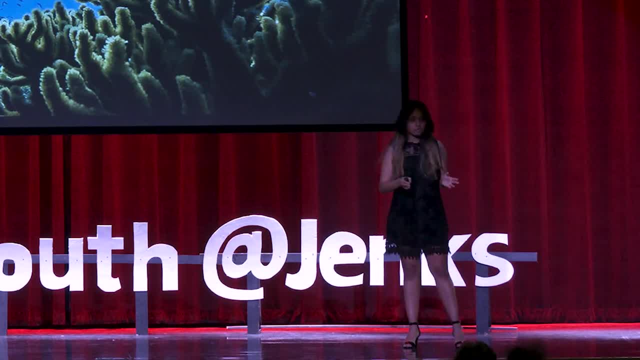 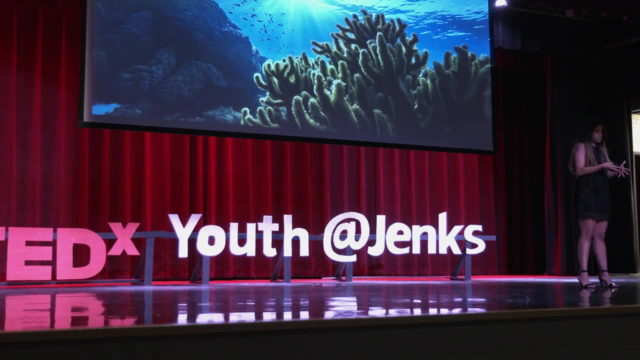 in Mr O'Horn's class and in my experiment I conducted ten trials that emitted different carbon dioxide levels into different aquariums And I put algae to have a photosynthetic organism into the aquarium and then I put a carbon dioxide to have carbon dioxide actually dissolve into the aquarium and my results showed. 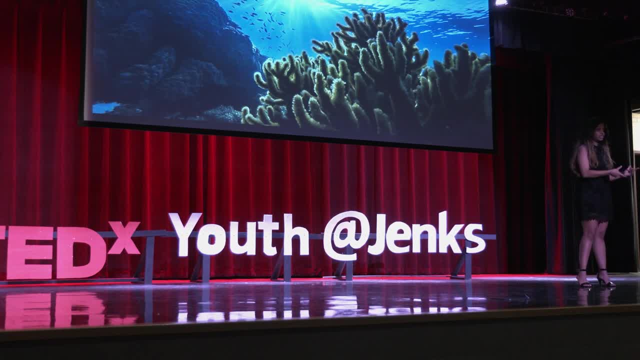 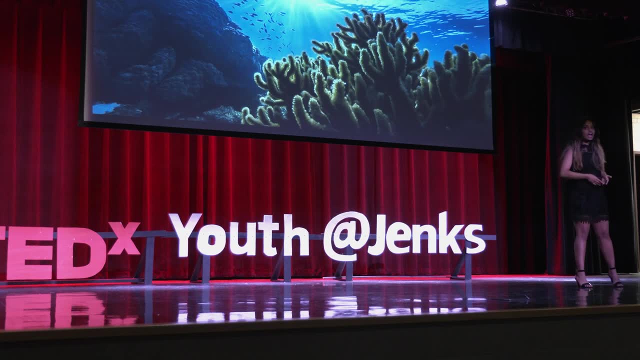 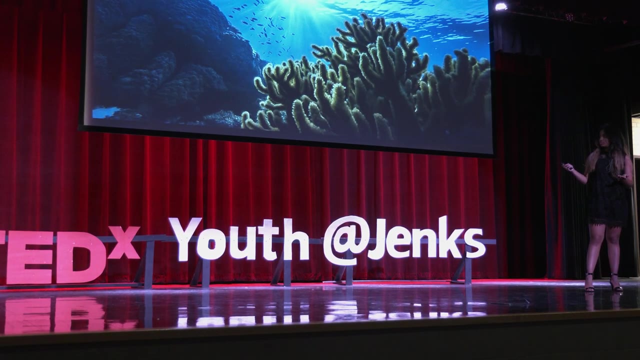 that the more carbon dioxide that gets in, submitted into the aquarium, the there is a more reduction in the pH of the ocean. so, as years go by, if I go back to this graph, okay, as years go by and as you can see, in 2100, the pH of the ocean. 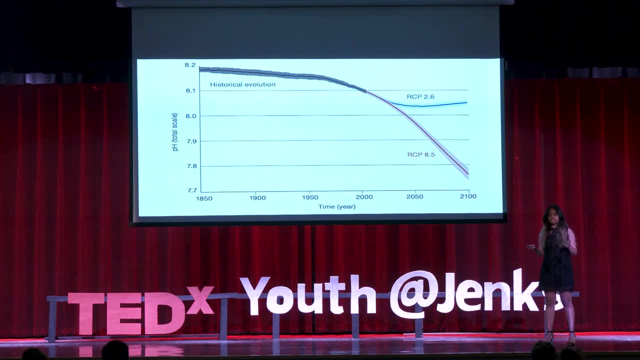 will be drastically reducing to an acidic level now. this is a major problem to marine life and ultimately affects everyone around us. thank you,